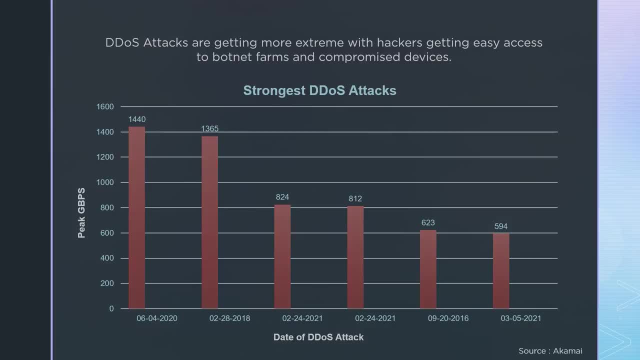 easy access to botnet farms and compromised devices. As can be seen in the graph, three of the six strongest DDoS attacks were launched in 2021, with the most extreme attack occurring just last year in 2020.. Lately, cybercriminals have been actively seeking out new services and protocols. 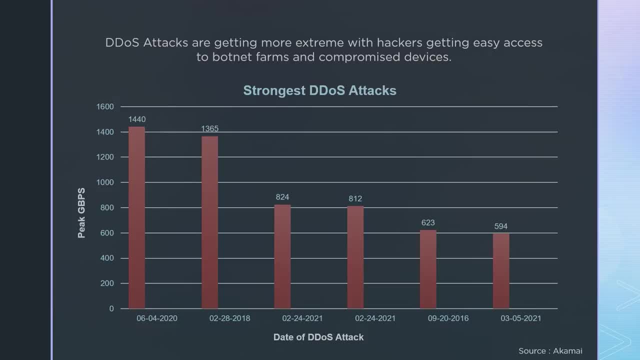 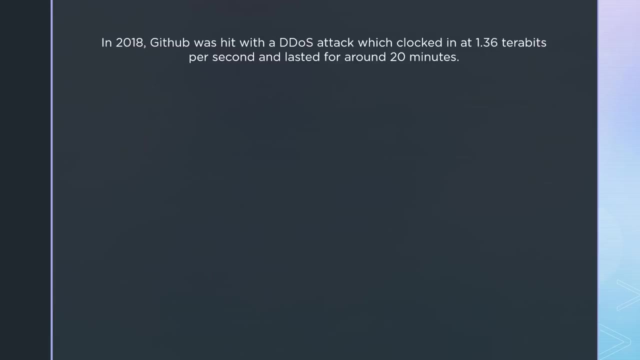 for amplifying these DDoS attacks. Active involvement with hacked machines and botnets allow further penetration into the consumer space, allowing much more elaborate attack campaigns. Apart from general users, multinational corporations have also had their fair share of problems. GitHub, a platform for software developers, was the target of a DDoS attack in. 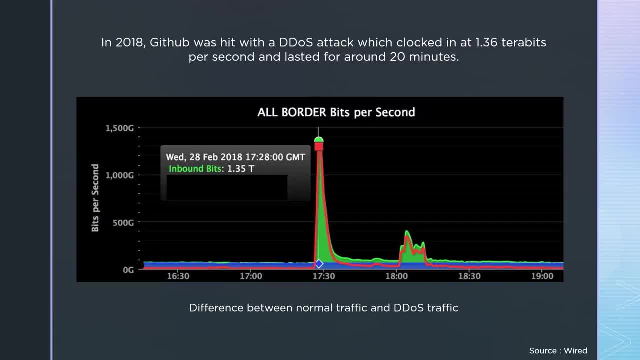 2018.. Widely suspected to be conducted by Chinese authorities, this attack went on for about 20 minutes, after which the systems were brought into a stable condition. It was the strongest DDoS attack to date. at the time, and made a lot of companies reconsider their security practices. 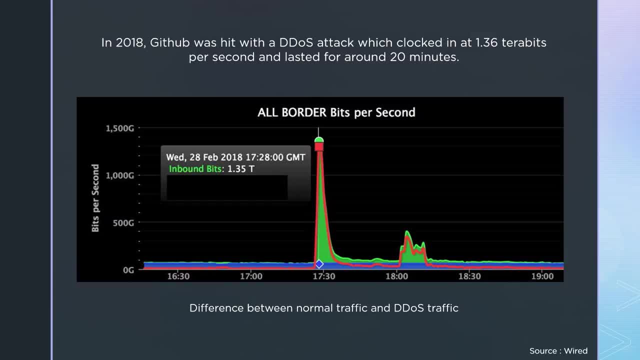 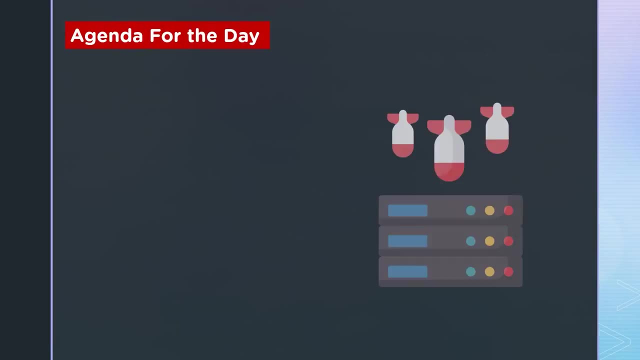 to combat such attacks. Even after years of experimentation, DDoS attacks are still at large and can affect anyone in the consumer and corporate space. Hey everyone, this is Baibab from Simply Learn, and welcome to this video on what is a DDoS attack. Let's take a look at the topics we will 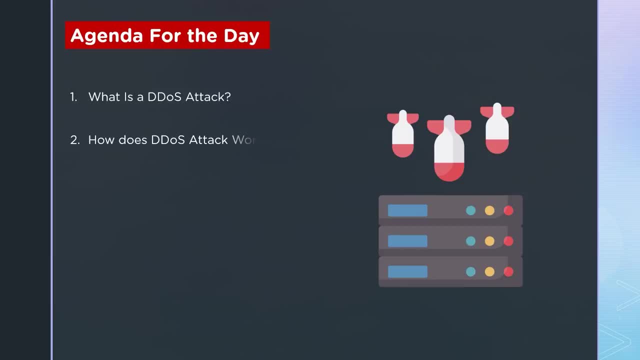 be covering today. We start by learning what is a DDoS attack and how it works on a face-by-face system. We learn about the distinct categories in DDoS attacks and the potential aim of hackers when they launch a DDoS attack campaign. We also look at some preventive measures that can be taken. 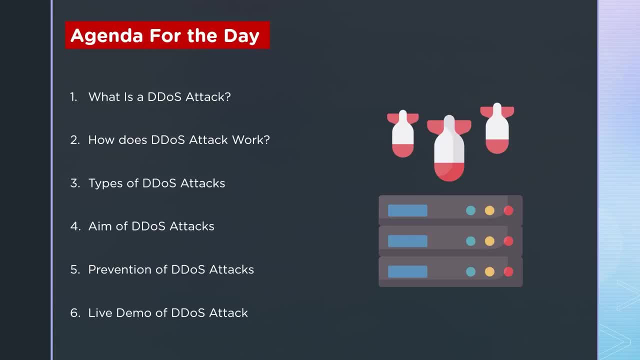 to protect oneself from these DDoS attacks. Finally, we have a demonstration of how such attacks can hamper the working of a server system using VMware and Parrot security operating system. But before moving forward, make sure you are subscribed to the Simply Learn YouTube channel. 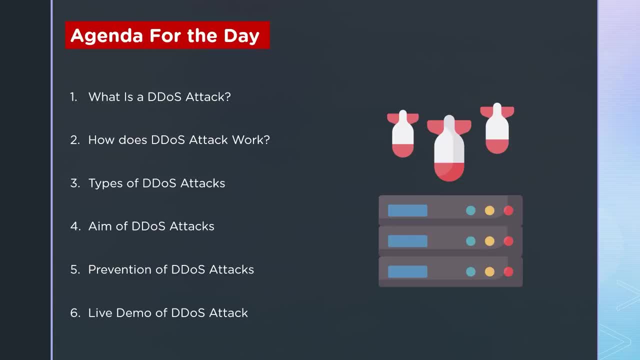 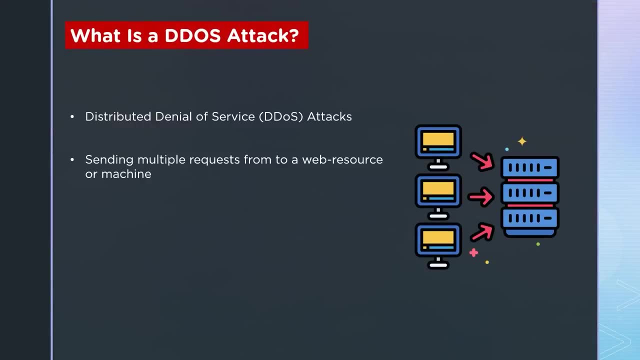 And don't forget to hit the bell icon to receive updates about more informative videos from our channel. So let's learn more about what is a DDoS attack. A distributed denial of service attack, or DDoS, is when an attacker or attackers attempt to make it impossible for a service to be delivered. 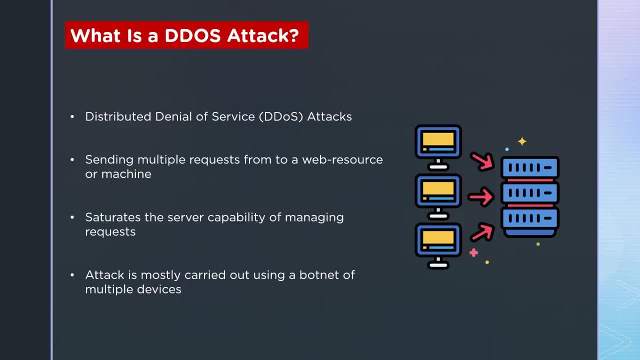 This can be achieved by thwarting access to virtually anything: servers, devices, services, networks, applications and even specific transactions within applications. In a DDoS attack, it's one system that is sending the malicious data or requests, A DDoS attack comes. 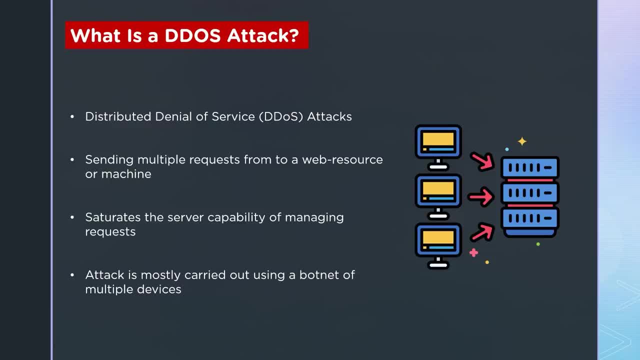 from multiple systems. Generally, these attacks work by drowning a system with requests for data. This could be sending a web server so many requests to serve a page that it crashes under the demand, or it could be a database being hit with a high volume of queries. The result is 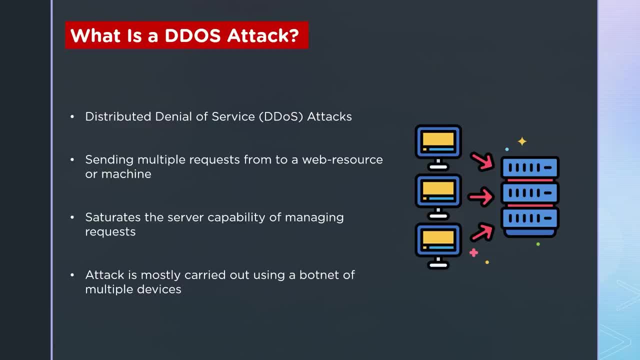 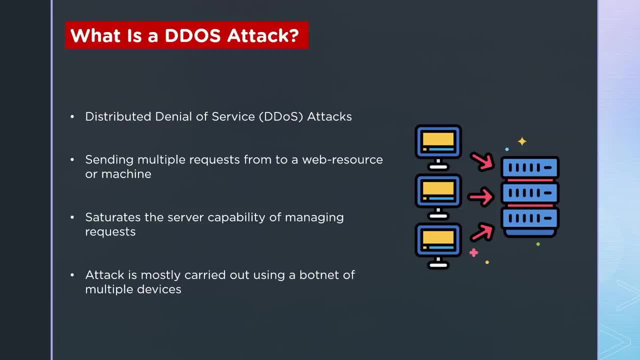 impact could range from a minor annoyance to a high volume of queries. The impact could range from disrupted services to experiencing entire websites, applications or even entire businesses taking offline. More often than not, these attacks are launched using machines in a botnet. A botnet is a. 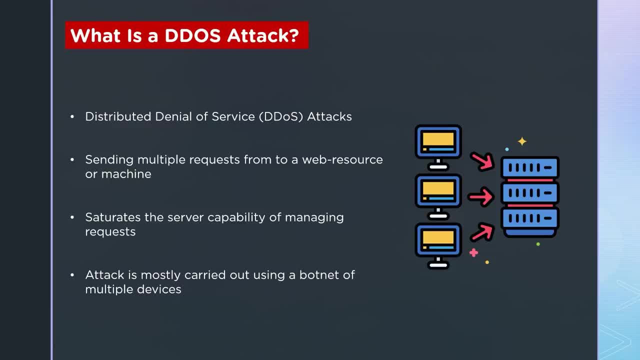 network of devices that can be triggered to send requests from a remote source, often known as the command and control center. The bots in the network attack a particular target, thereby hiding the original perpetrator of the DDoS campaign. But how do these devices come under control In the 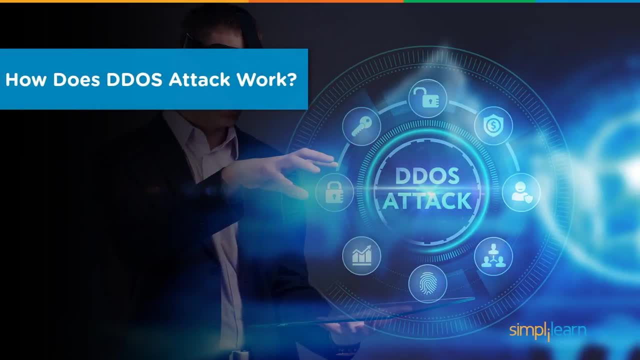 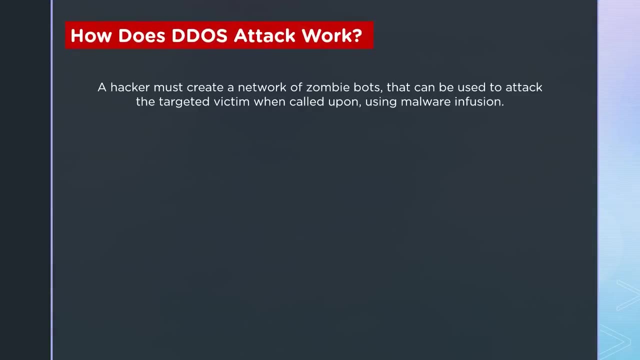 botnet. what are the requests being made to the web servers? Let's learn more about these and how DDoS attack work. A DDoS attack is a two-phase process. In the first phase, a hacker creates a botnet of devices. Simply put, a vast network of computers are hacked via malware, ransomware or 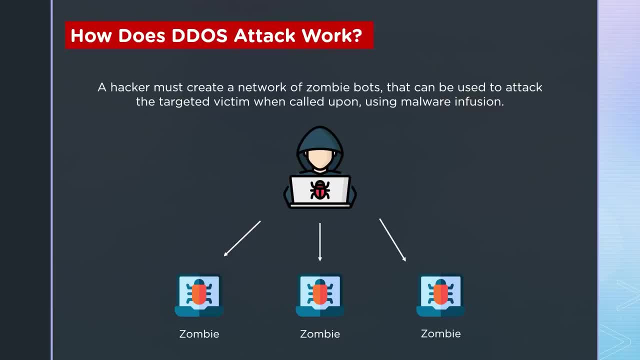 just simple social engineering. These devices become a part of the botnet, which can be triggered anytime to start bombarding a system or a server. The botnet is a device that can be triggered any time to start bombarding a system or a server. The botnet is a device that can be triggered anytime to 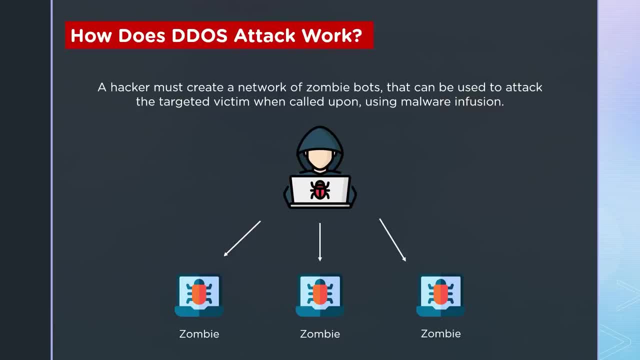 start bombarding a system or a server. The botnet is a device that can be triggered anytime to start bombarding a system or a server on the instruction of the hacker that created the botnet. The devices in these networks are called bots or zombies. In the second phase, a particular target is: 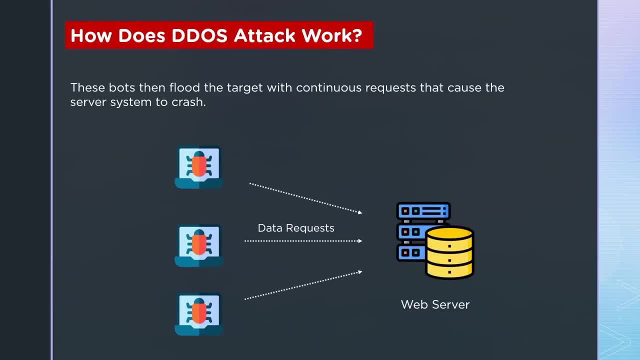 selected for the attack. When the hacker finds the right time to attack all the zombies in the botnet network, send these requests to the target, thereby taking up all the server's available bandwidth. These can be simple ping requests or complex attacks like SYN flooding and UDP flooding. 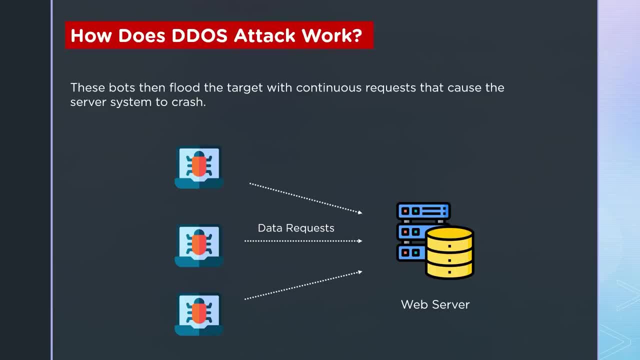 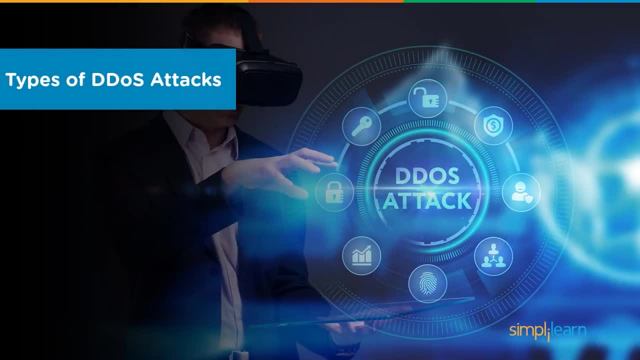 The aim is to overwhelm them with more traffic than the server or the network can accommodate. The goal is to render the website or service inoperable. There is a lot of wiggle room when it comes to the type of DDoS attack a hacker can go. 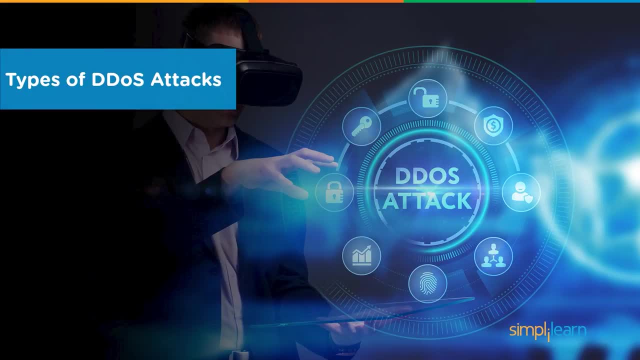 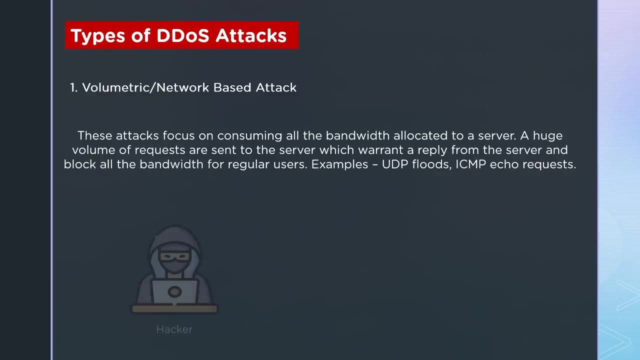 with. Depending on the target's vulnerability, we can choose one of the three broad categories of DDoS attacks. Volume based attacks use massive amounts of bogus traffic to overwhelm a resource. It can be a website or a server. They include ICMP, UDAP and spoofed packet flood attacks. 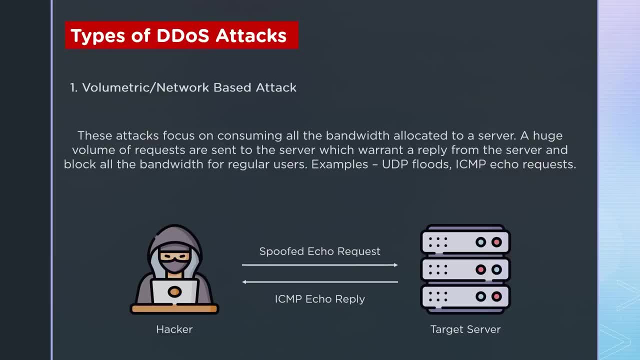 The size of volume based attack is measured in bits per second. These attacks focus on clogging all the available bandwidth for the server, thereby cutting the supply short. Several requests are sent to the server, all of which warrant a reply, thereby not allowing. 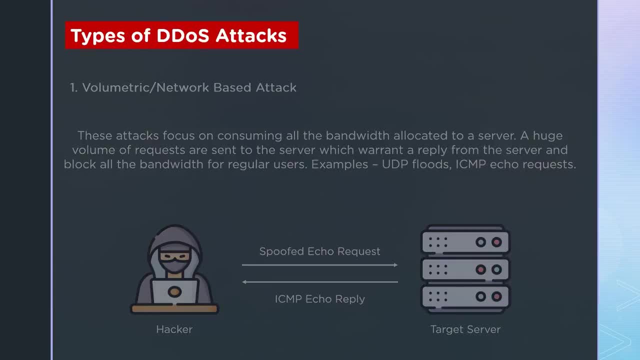 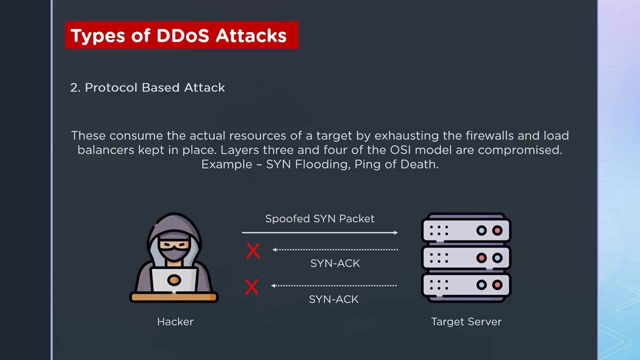 the target to cater to the general legitimate users. Next, we have the protocol level attacks. These attacks are meant to consume essential resources. They exhaust the load balancers and firewalls which are meant to protect the system against the DDoS attacks. 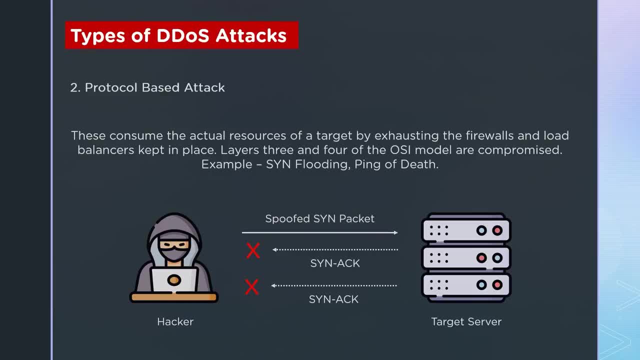 These protocol attacks include SYN floods and smurf DDoS, among others, and the size is measured in packets per second. For example, in an SSL handshake server replies to the hello message sent by the hacker, which will be the client in this case. 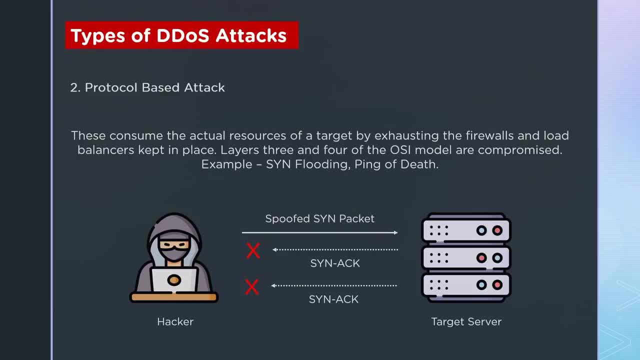 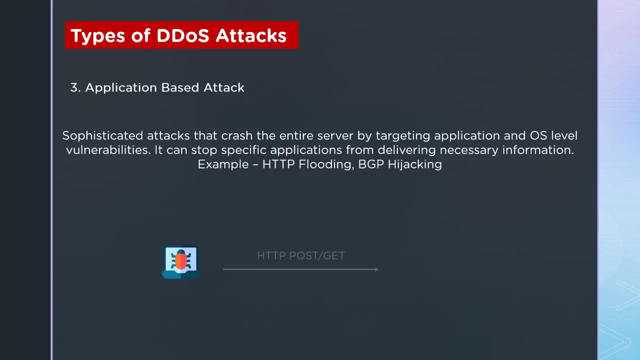 But since the IP is spoofed and leads nowhere, the server gets stuck in an endless loop of sending the acknowledgement without any end in sight. Finally, we have the application level attacks. Application layer attacks are conducted by flooding applications with maliciously crafted requests. 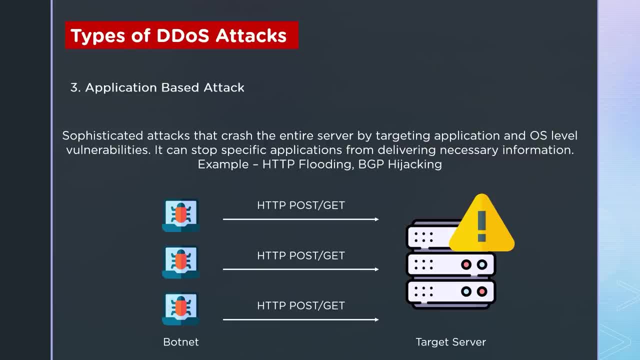 The size of application layer attacks is measured in requests per second. These are relatively sophisticated attacks that target the application and operating system level vulnerabilities. They prevent the specific applications from delivering necessary information to users and hog the network bandwidth up to the point of a system crash. 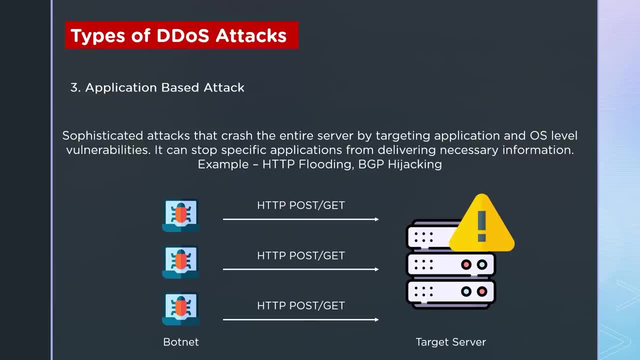 Examples of such an attack are HTTP flooding and BGP hijacking. A single device can request data from a server using HTTP POST or GET without any issues. However, when the requisite botnet is instructed to bombard the server with thousands of requests, the database bandwidth gets jammed and it eventually becomes unresponsive and unusable. 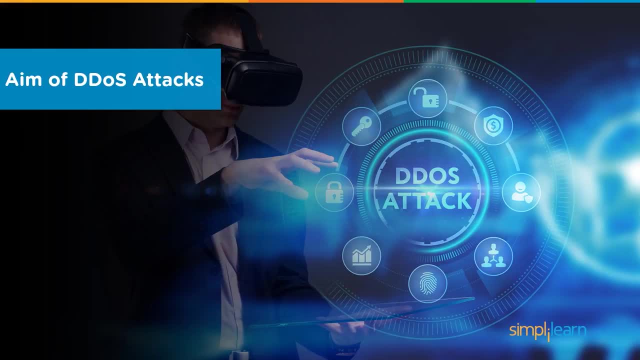 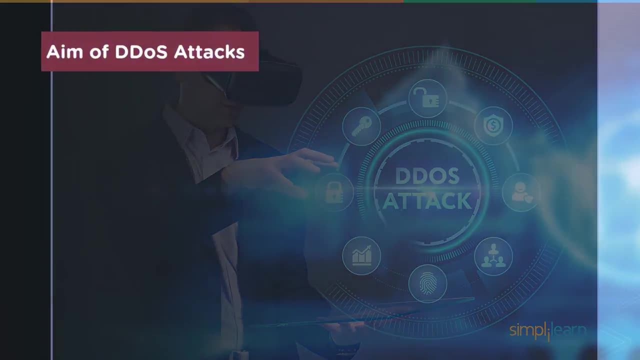 But what about the reasons for such an attack? There are multiple lines of thought as to why a hacker decides to launch a DDoS attack on unsuspecting targets. Let's take a look at a few of them. The first option is to gain a competitive advantage. 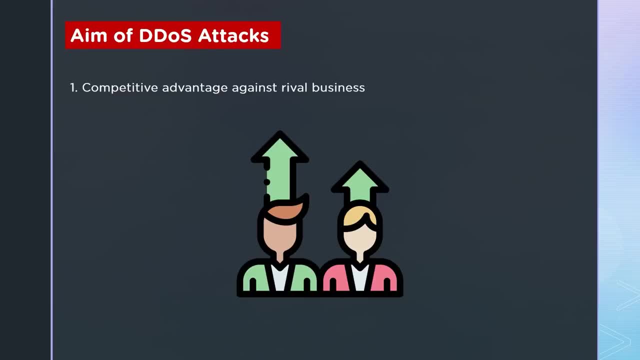 Many DDoS attacks are conducted by hacking communities against rival groups. Some organizations hire such communities to stagger their rival's resources at a network level to gain an advantage in the playing field. Since being a victim of a DDoS attack indicates a lack of security, the DDoS attack can be 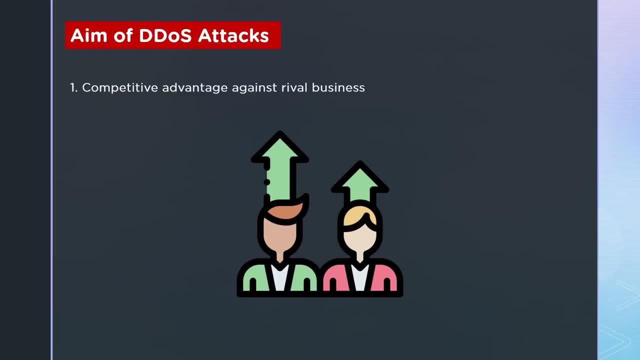 used as an excuse to attack The reputation of such a company takes a significant hit, allowing their rivals to cover up some ground. Secondly, some hackers launch these DDoS attacks to hold multinational corporations at ransom. The resources are jammed and the only way to clear the way is if the target company 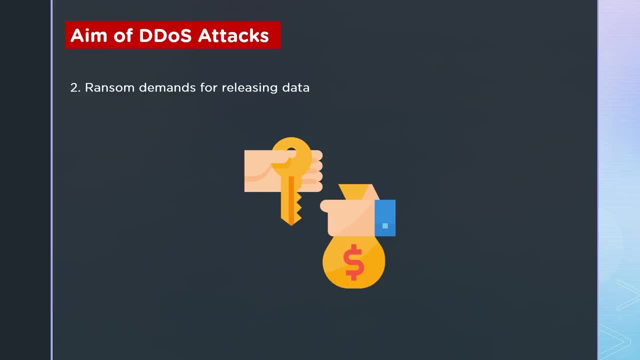 agrees to pay a designated amount of money to the hackers. Even a few minutes of inactivity is detrimental to a company's reputation in the global market, and it can cause a spiral effect both in terms of market value and in terms of the product security index. 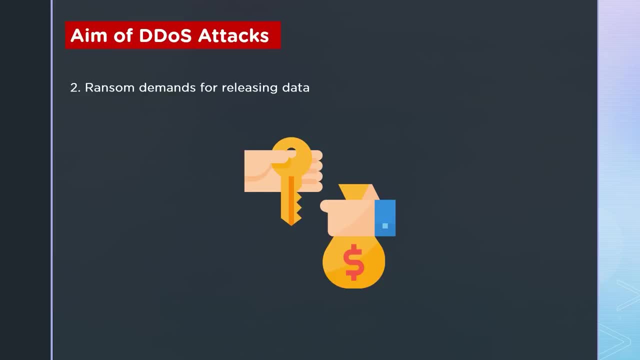 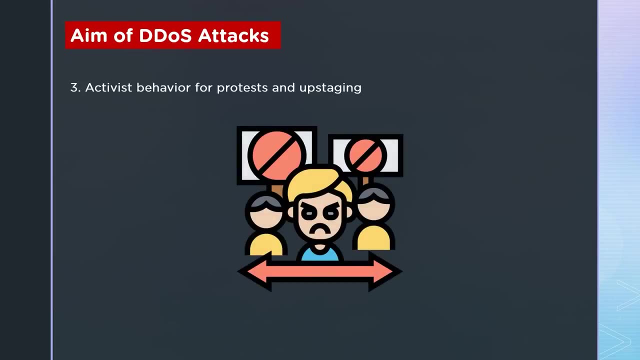 Most of the time, a compromise is reached and the resources are freed after a while. DDoS attacks have also found use in the political segment. Certain activists tend to use DDoS attacks to voice their opinion. Spreading the word online is much faster than any local rally or forum. 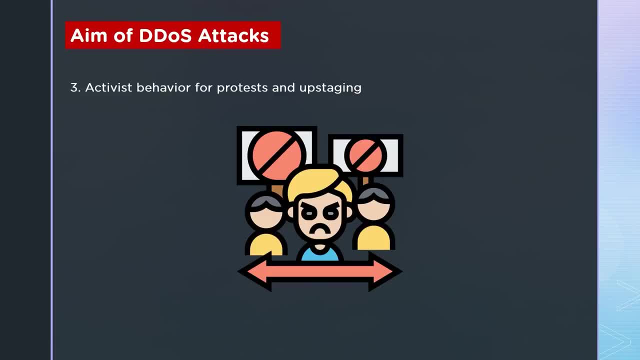 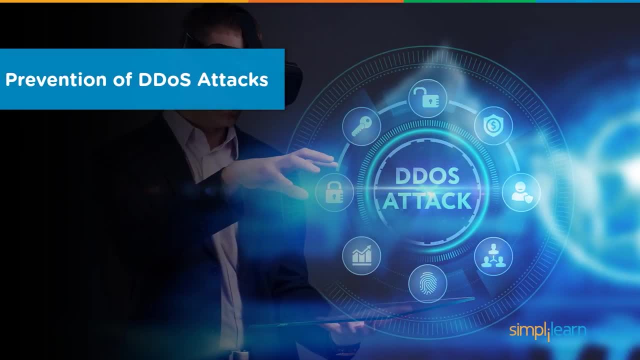 Primarily political, these attacks also focus on online communities, ethical dilemmas or even protests against corporations. Let's take a look at some of these attacks. The first one is DDoS. Let's look at a few ways that companies and individuals can protect themselves against. 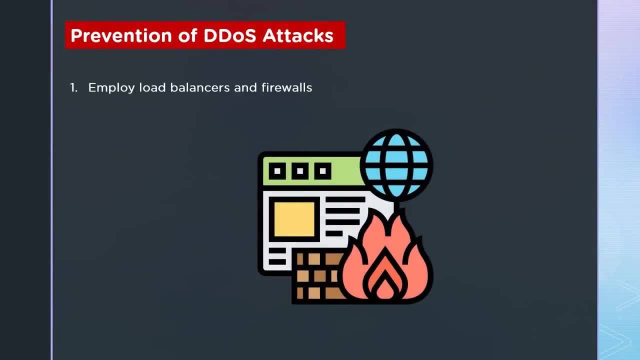 DDoS attacks, The company can employ load balancers and firewalls to help protect the data from such attacks. Load balancers reroute the traffic from one server to another in a DDoS attack. This reduces the single pointer failure and adds resiliency to the server data. 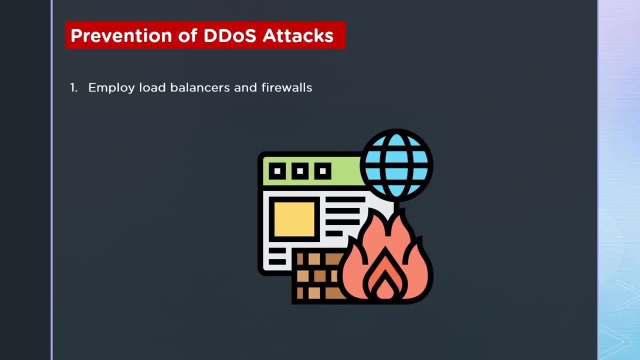 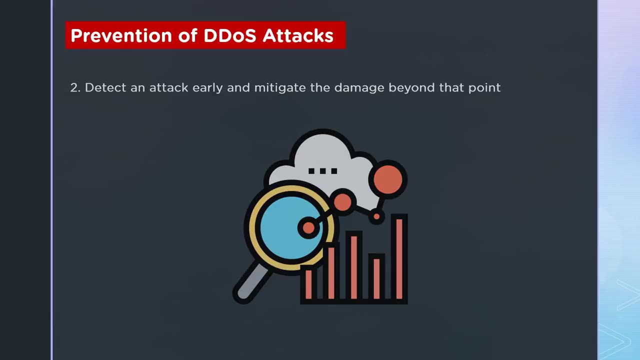 A firewall blocks unwanted traffic into a system and manages the number of requests made at a definite rate. It checks for multiple attacks from a single IP and occasional slowdowns to detect a DDoS attack in action. Early detection of a DDoS attack goes a long way in recovering the data lost in such an 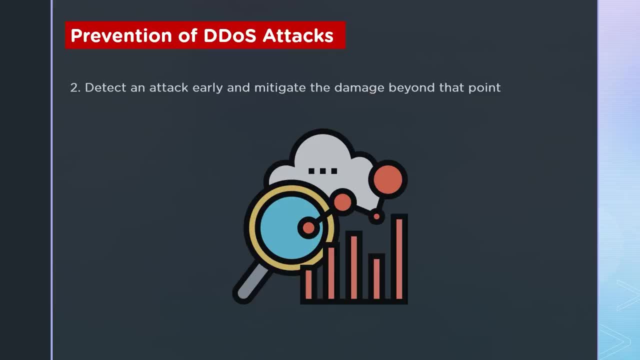 event. Once you've detected the attack, you'll have to find a way to respond. For example, you'll have to work on dropping the malicious DDoS traffic before it reaches your server, so that it doesn't throttle and exhaust your bandwidth. 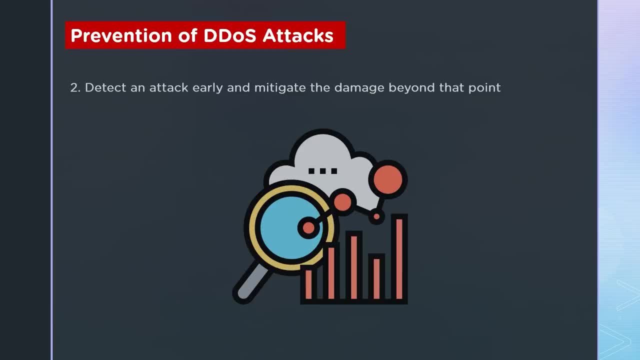 Here's where you'll filter the traffic so that only legitimate users can access the DDoS traffic. The DDoS attack can be detected by a single IP. If it's on the server's IP, your system will automatically help you to get the DDoS. 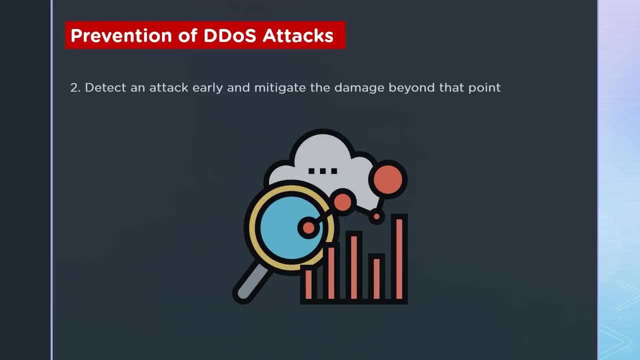 attack. By intelligent routing you can break the remaining traffic into manageable chunks that can be handled by your cluster resources. The most important stage in DDoS mitigation is where you'll look for patterns of DDoS attacks and use those to analyze and strengthen your mitigation techniques. 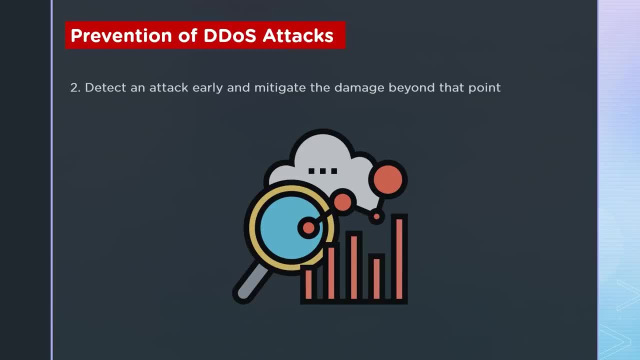 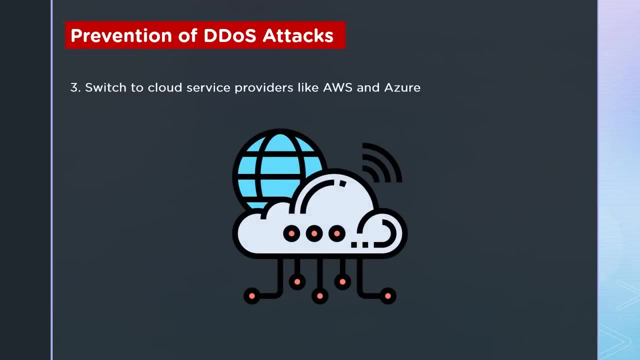 For example, blocking an IP that's repeatedly found to be offending is the first step. This is also where you'll have to take some time to define all your DDoS attacks. This is the most important step in DDoS mitigation. Cloud providers like Amazon Web Services and Microsoft Azure, who offer high levels of cyber security, including firewalls and threat monitoring software, can help protect your assets and network from DDoS criminals. 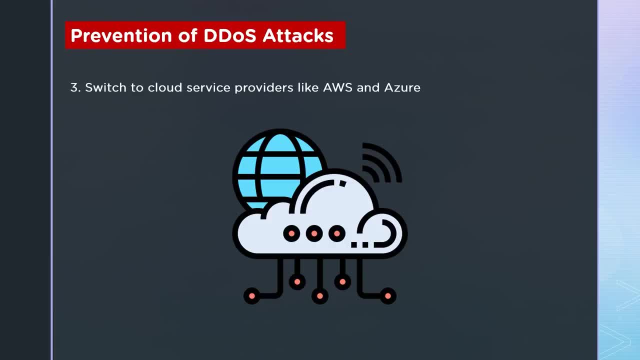 The cloud also has greater bandwidth than most private networks, so it is likely to fail if under the pressure of increased DDoS attacks. Additionally, reputable cloud providers offer network redundancy- duplicating copies of your data systems and equipment, so that, if your service becomes corrupted or unavailable due to a DDoS attack, you can switch to a secure access on backed-up versions without missing a beat. 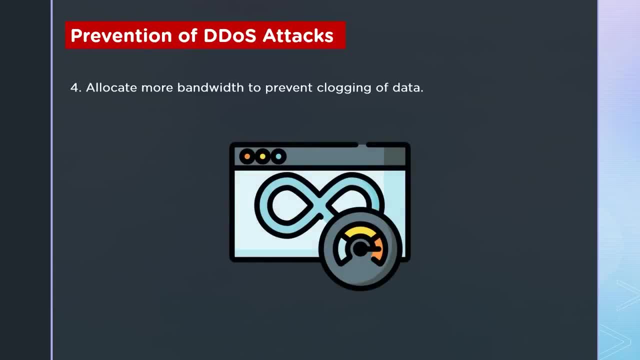 One can also increase the amount of bandwidth available to a host server being targeted. Since DDoS attacks fundamentally operate on the principle of overwhelming systems with heavy traffic, simply provisioning extra bandwidth to handle unexpected traffic spikes can provide a measure of protection. This solution can prove expensive, as a lot of that bandwidth is going to go unused most of the time. 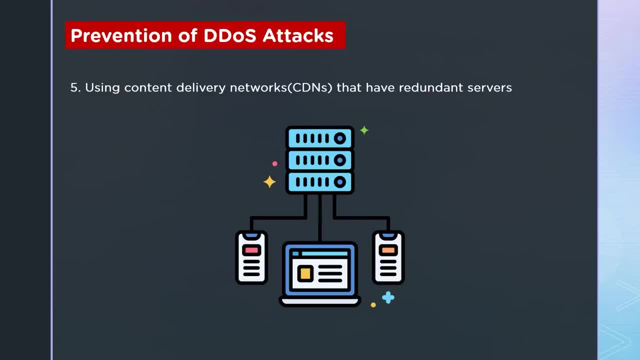 A Content Delivery Network, or a CDN, distributes your content and boosts performance by minimizing the distance between your resources and end users. It stores the cached version of your content in multiple locations and this eventually mitigates DDoS attacks by avoiding the risk of DDoS attacks. 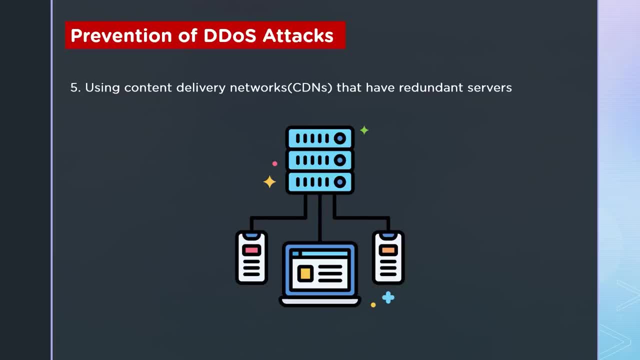 It also provides a single point of failure when the attacker is trying to focus on a single target. Popular CDNs include Akamai, CDN, Cloudflare, AWS, CloudFront, etc. Let's start with our demo regarding the effects of DDoS attacks on a system. 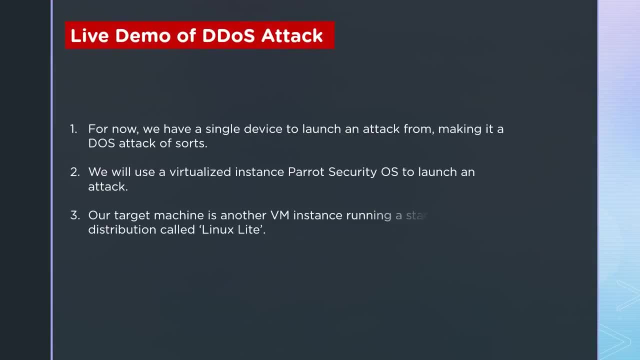 For our demo we have a single device that will attack a target, making it a DDoS attack of sorts. Once a botnet is ready, multiple devices can do the same and eventually emulate a DDoS attack. To do so we will use the virtualization software called VMWare, with an instance of Parrot Security operating system running. 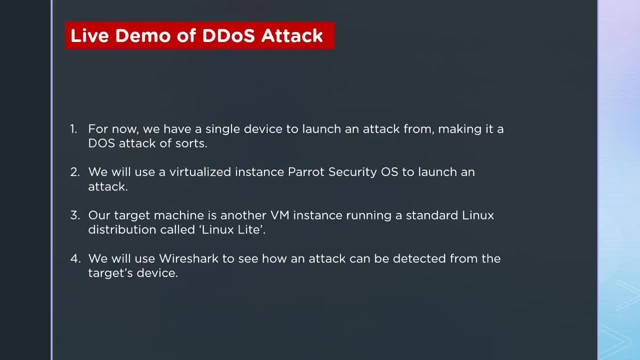 For a target machine. we will be running another VMWare instance of a standard Linux distribution known as Linux Lite In a target device. we can use Wireshark to determine when the attack begins and see the effects of the attack accordingly. 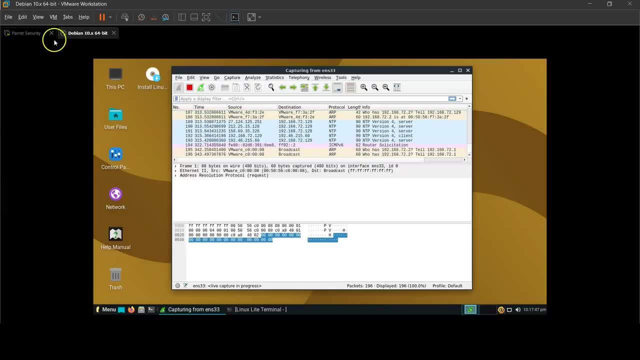 This is Linux Lite, which is our target machine, And this is Parrot Security, which is our target machine, And this is Parrot Security, which is our target machine. This is a DDoS attack that is used by the hacker when trying to launch a DDoS attack. 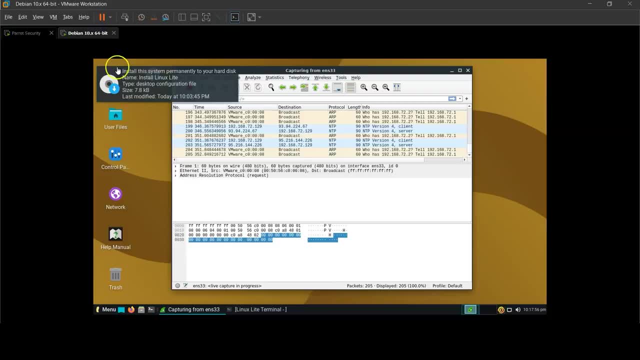 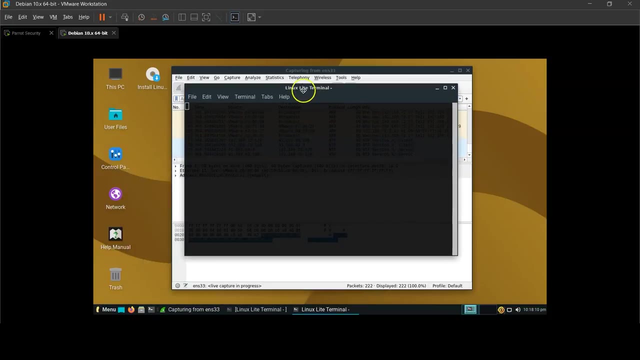 This is just one of the distros that can be used To launch the attack. we must first find the IP address of our target. To find the IP address, we open the terminal, We use the command ifconfig And here we can find the IP address. 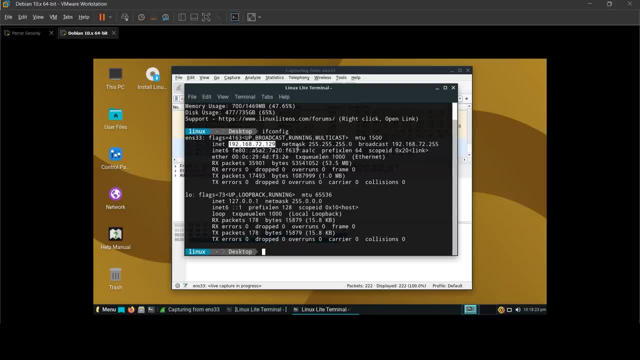 now remember, we're launching this attack in vmware. now the both the instances of parrot security and linux lite are being run on my local network, so the address that you can see here is 192.168.72.129, which is a private address. this ip cannot be accessed from outside the network. basically. 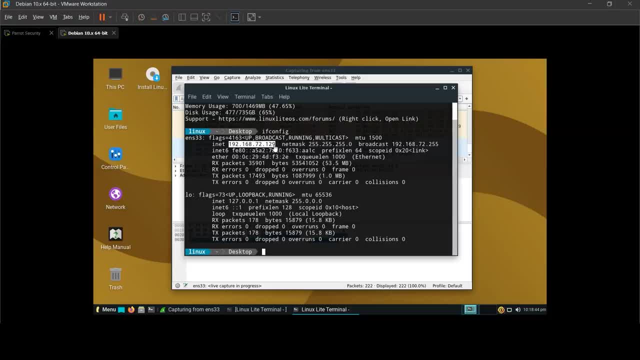 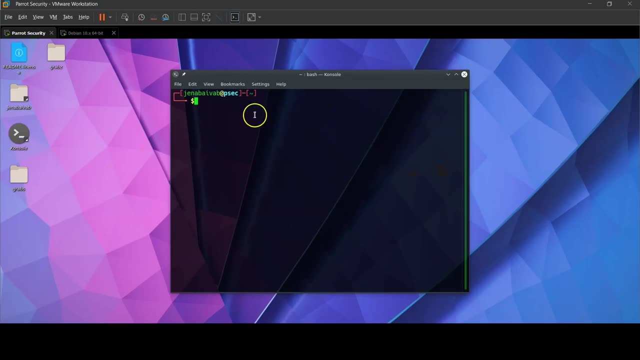 anyone who is not connected to my wi-fi. when launching attacks with public servers or public addresses, it will have a public ip address that does not belong to the 192.168 subnet. once we have the ip address, we can use a tool called hping3. 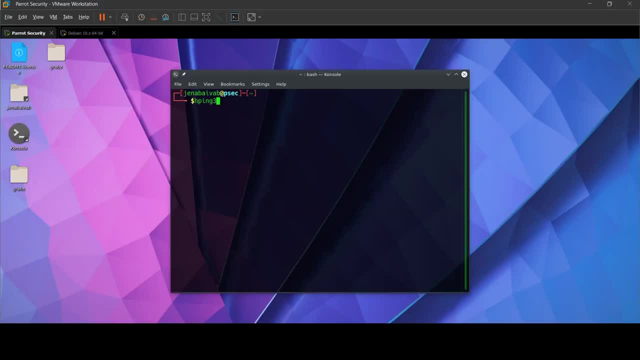 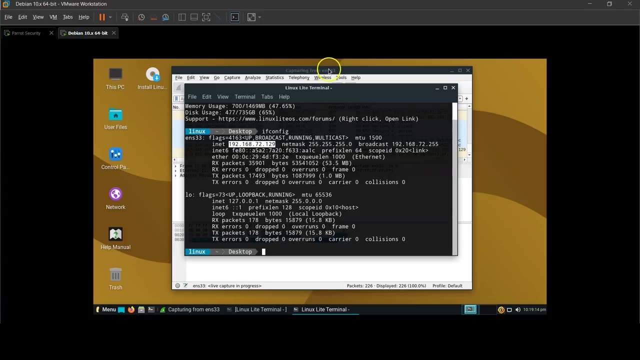 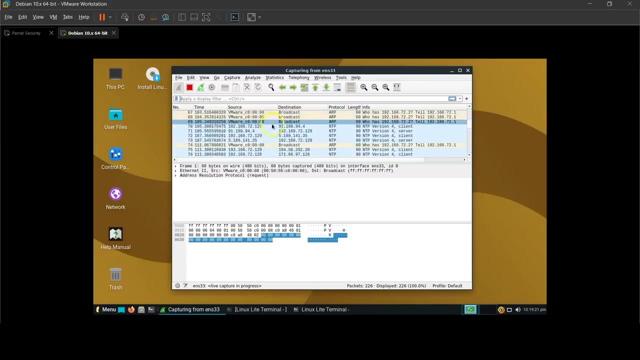 hping3 is an open source packet generator and analyzer for the tcp ip protocol. to check what are the effects of an attack, we will be using wireshark. wireshark is a network traffic analyzer. we can see whatever traffic that is passing through the linux lite. 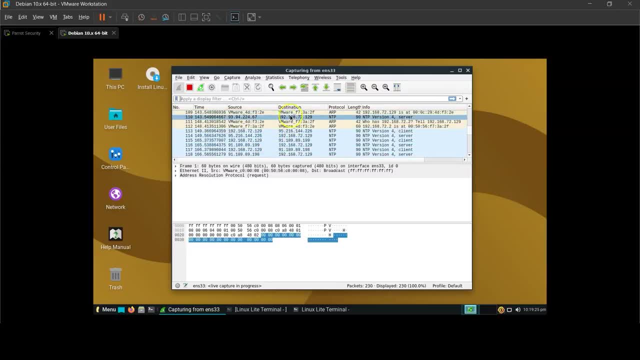 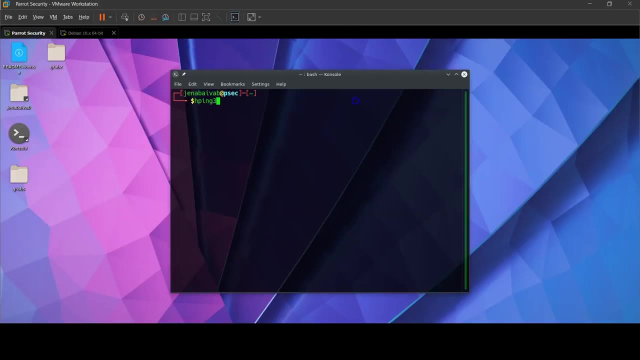 distro is being displayed over here with the ip address, the source ip and the destination ip as to where the request is being transferred to once we have the dos attack launched. you can see the results coming over here from the source ip, which will be parrot security. 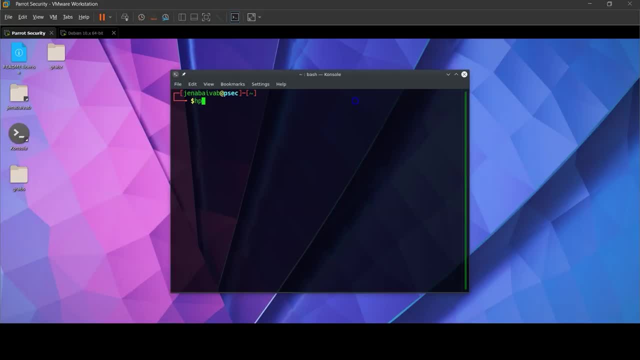 now, to launch the hping3 command, we need to give sudo access to the console, which is the root access for the console. now we have the root access for the console, the hping3 command will have a few arguments to go with it, which are, as you can see on the screen, minus s and a flood hyphen v. 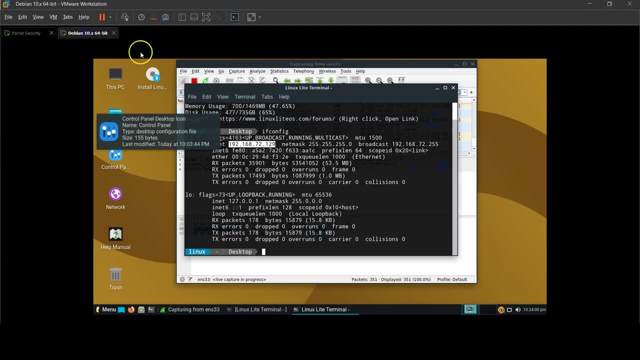 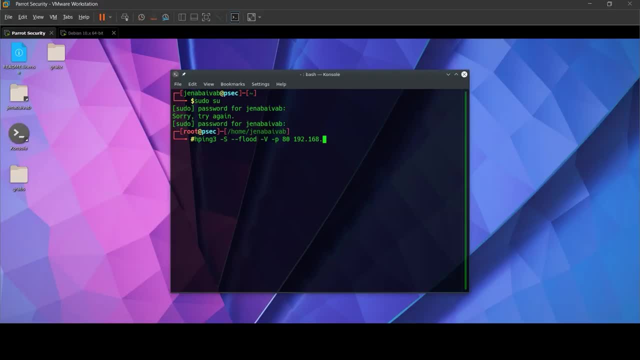 hyphen p18 and the ip address of the target, which is 192.168.7.1. In this command we have a few arguments, such as the "-s" which specifies SYN packets. Like in an SSL handshake, we have the SYN request that the client sends to the server. 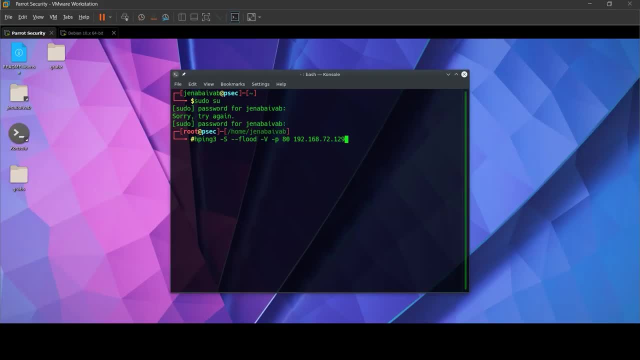 to initiate a connection. The "-flood" aims to ignore the replies that the server will send back to the client in response to the SYN packets. Here the Parrot Security OS is the client and Linux Lite being the server. "-v" stands for verbosity, as in, where we will see some output when the requests are. 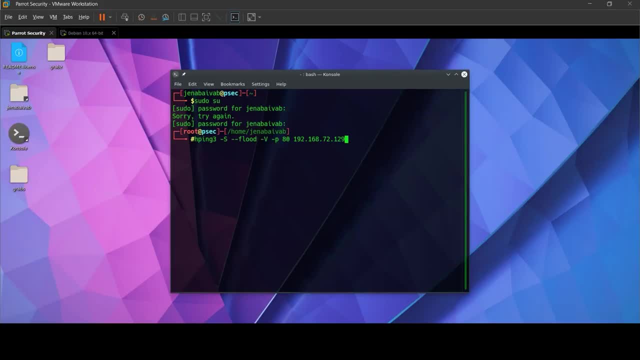 being sent. The "-p80" stands for port 80, which we can replace the port number if we want to attack a different port. And finally, we have the IP address of our target As of right now if we check via Shark. 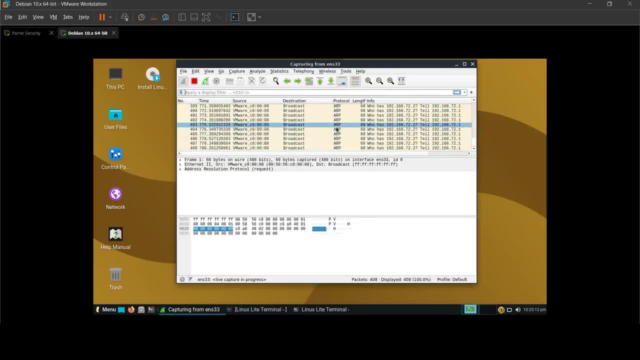 It is relatively clear, and there is no indication of a DDoS attack incoming Now. once we launch the attack over here, we can see the requests coming in from this IP, which is 192.168.72.128.. Till now, even if the network is responsive, and so is Linux Lite, the requests keep on. 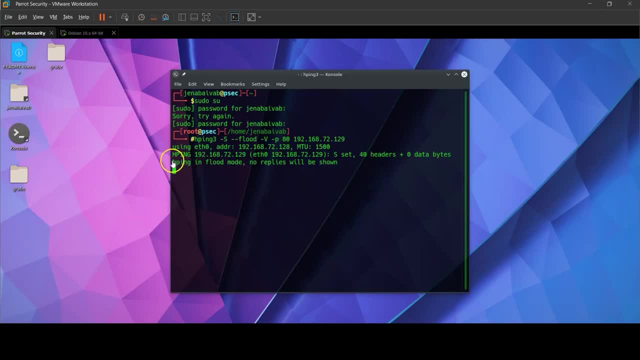 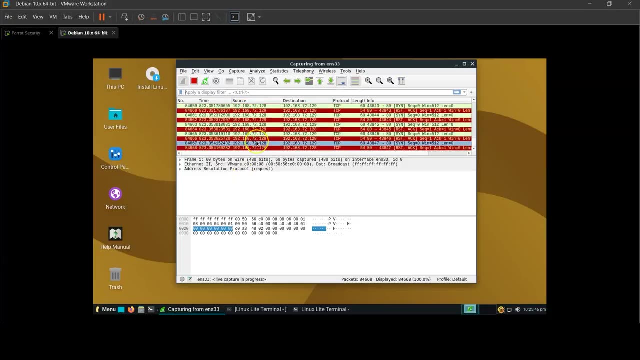 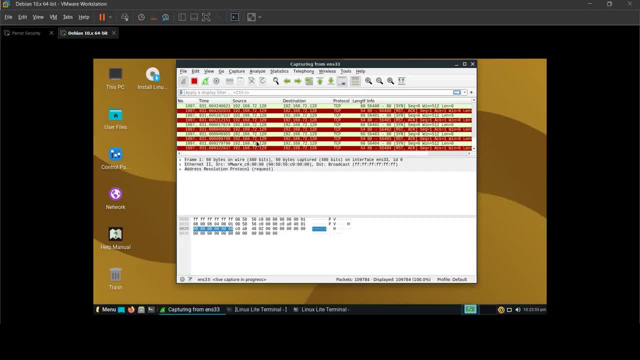 Now remember, Linux Lite is a distro that can focus onthat serves as a backend. Now remember, Linux Lite is a distro and such Linux distros are served as backend to many servers across the world. For example, a few seconds have passed from the attack. 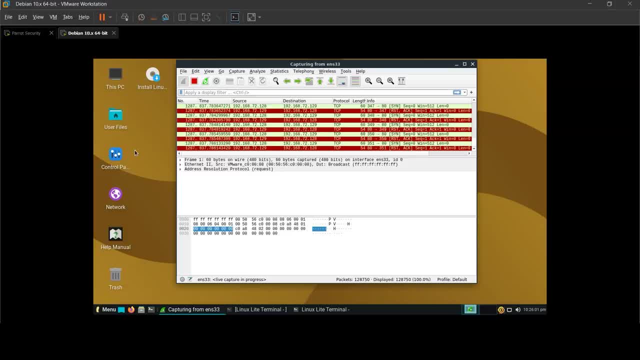 Now the system has become completely responsive. This has happened due to the huge number of requests that came from Parallel Security. You can see, whatever I press, nothing is responded. even the wireshark has stopped capturing new requests because the CPU usage right now is completely 100% and at this point of time, anyone who is trying to request some information from 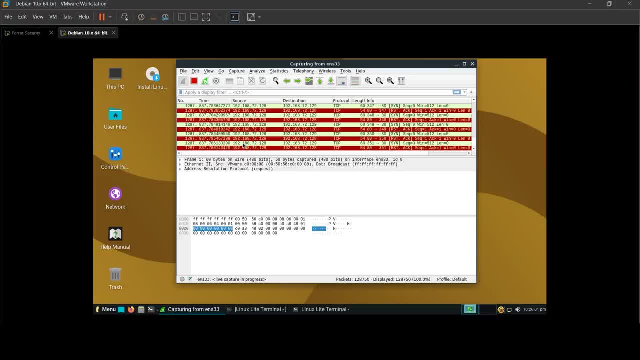 this Linux distro, or where this Linux distro is being used as a backend for a server or a database, cannot access anything else. The system has completely stopped responding and any request, any legitimate request from legitimate users, will be dropped Once we stop the attack over here. 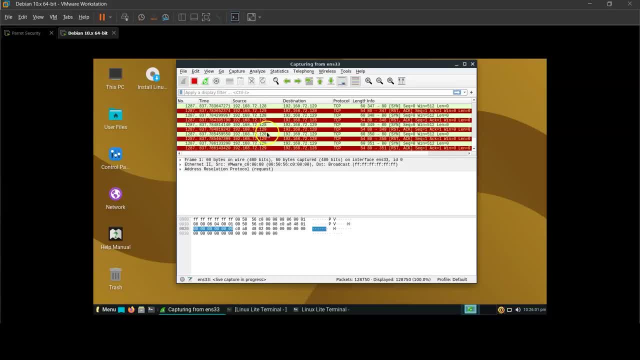 it takes a bit of time to settle down. Now, remember, it's still out of control, but eventually the traffic dies down and the system regains its strength. It is relatively easy to gauge right now the effect of a DOS attack. Now remember this: Linux Lite is just a VM instance. 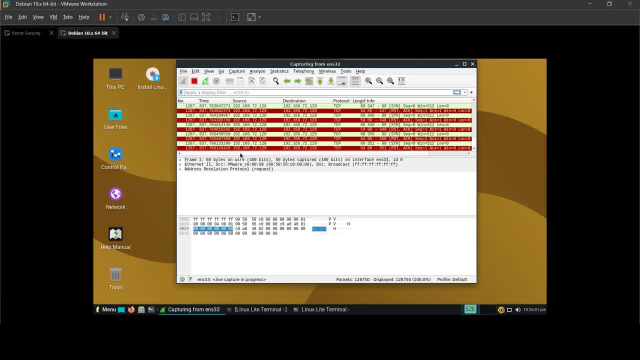 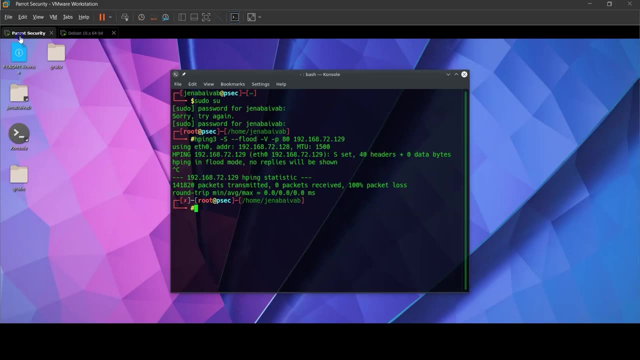 Actual website servers and web databases. they have much more bandwidth and are very secure and it is tough to break into. That is why we cannot use a single machine to break into them. That is where a DDoS attack comes into play. What we did right now is a DOS attack. 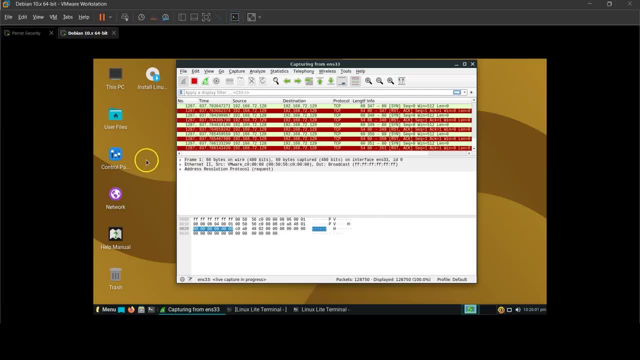 as in, a single system is being used to penetrate a target server using a single request. Now, when a DDoS attack multiple systems, such as multiple security instances or multiple zombies or bots in a botnet network, can attack a target server to completely shut down the machine and drop any legitimate requests. 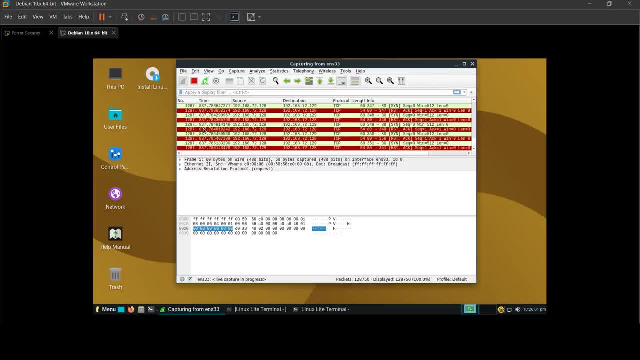 thereby rendering the service and the target completely unusable and inoperable. As a final note, we would like to remind that this is for educational purposes only and we do not endorse any attacks on any one domains. Only test this on servers and networks that you have.